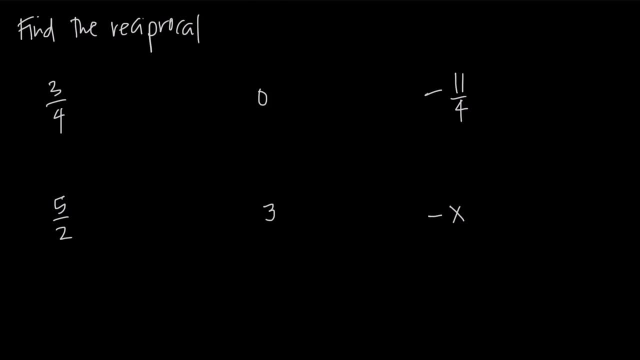 In this video, we're going to be talking about reciprocals, and the only thing you need to know about reciprocals is that the reciprocal of something is whatever. you can multiply this thing by in order to make it equal to 1.. The reciprocal is also called the multiplicative. 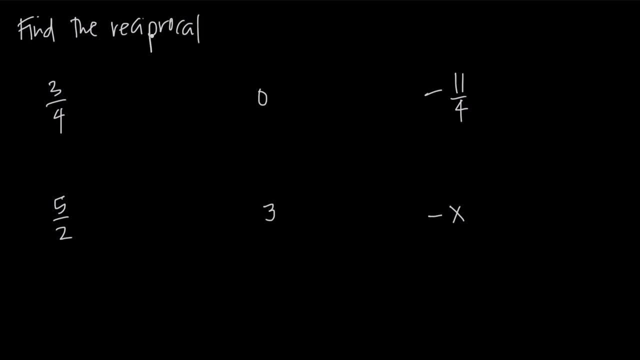 inverse, but of course we never use that term when we could just use the term reciprocal, because it's a lot easier to say. So what do we have to multiply by 3 over 4 in order to get 1?? Well, in fact it's just as easy as flipping this fraction upside down. So the 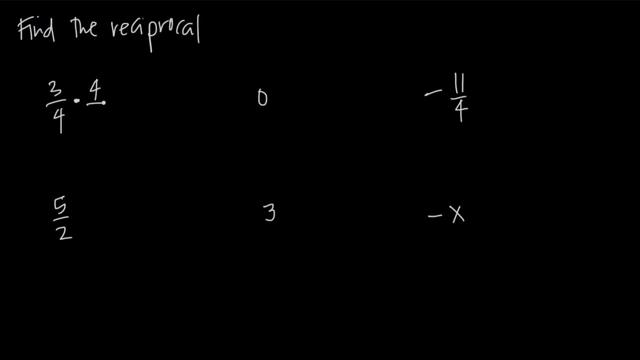 denominator is going to become the numerator and the numerator is going to become the denominator. So we just flipped the place of the numerator and the denominator. We flipped this straight upside down, flipped their places and now, when we multiply straight across 3 times, 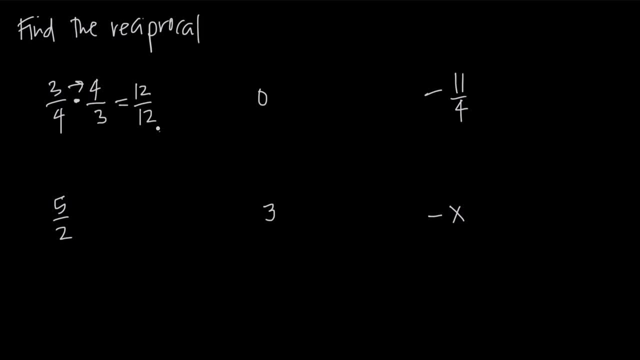 4 gives me 12.. 4 times 3 gives me 12, and anything over itself, we know, is 1.. So 12 over 12 is equal to 1.. So 4 thirds was what I had to multiply by 3 fourths in order to get 1.. 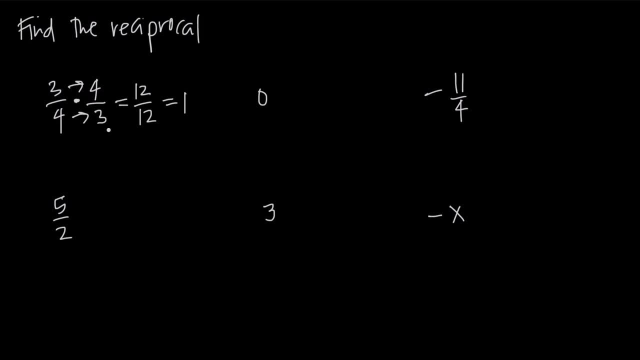 And that's always going to be the case, except GENERES. FOR EXAMPLE, When you're onto a page that has lots of candidates and it's easy for you to knit, we have 0, and we'll talk about that in a second. But in order to find the reciprocal, which 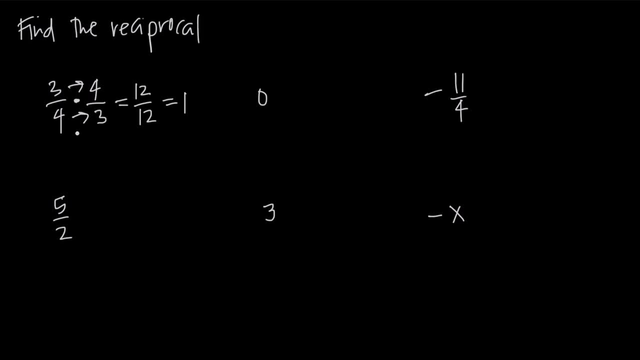 is whatever you have to multiply by in order to get 1, you just flip this upside down. So if we have 5 over 2, we just flip it upside down and we can say that the reciprocal is 2 fifths. So our reciprocal is going to be 2 fifths, just like our reciprocal was 4 thirds. 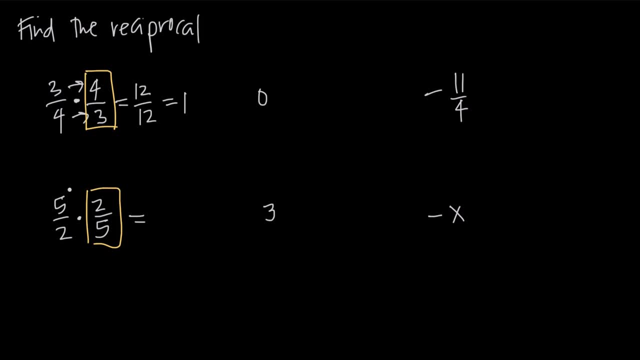 And we can prove that 2 fifths is the reciprocal by multiplying straight across. 5 times 2 is 10, 2 times 5 is 10, 10 over 10 is equal to 1.. So when we multiply by 2 fifths, we get: 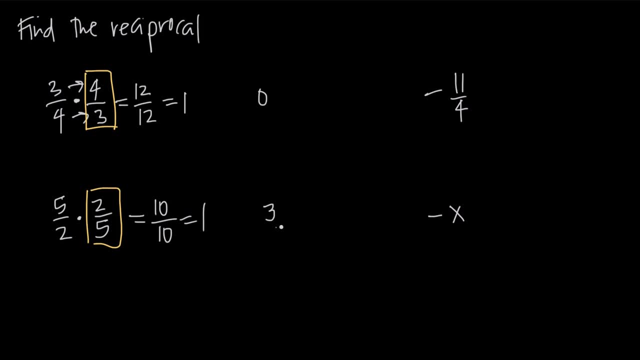 1, so we know that 2 fifths is the reciprocal. Now what happens when we try to find the reciprocal of 3?? Well, before, when we were dealing with a fraction, it was really easy because we just swapped the places of the numerator and the denominator. What happens when we just 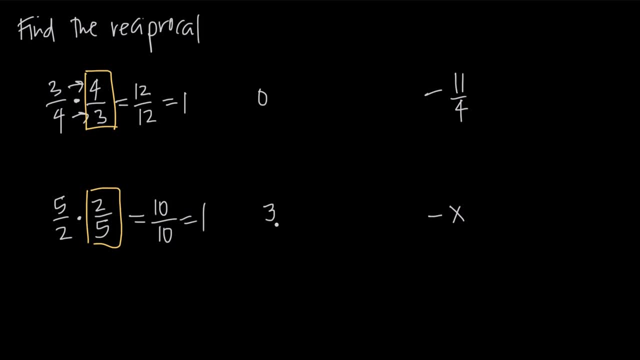 have a whole number. Well, in that case, we remember that this is still a fraction. 3 is actually 3 over 1, and now we have a fraction. We flip the fraction upside down and we get 1 over 3.. 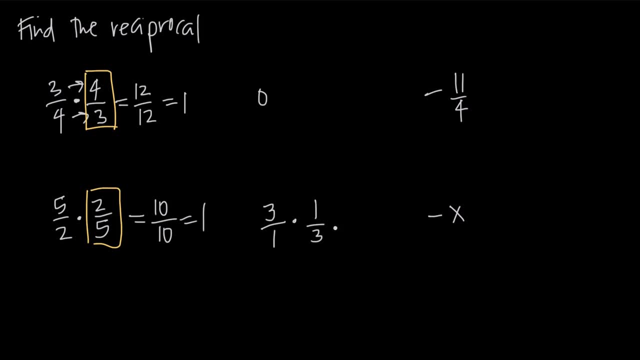 So the numerator becomes the denominator and the denominator becomes the numerator. and we say: 3 times 1 is 3, and 1 times 3 is 3, and 3 over 3 is 1, so we can say that 1 third is our reciprocal. 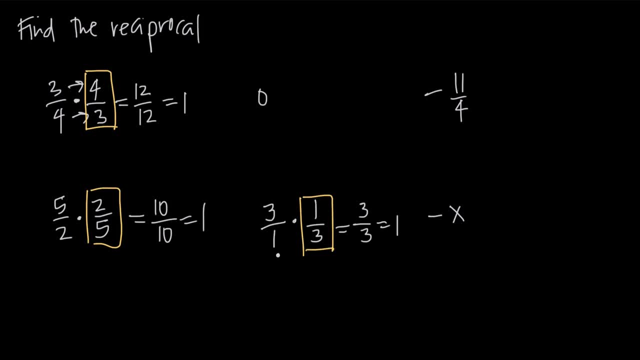 So when you have a whole number, when you just have 3, you make sure that you say 3 over 1, then you flip it upside down and you get the reciprocal. Now how does that apply when we have 0?? Well, you might think I can say this is 0 over 1, because 0 over 1 is. 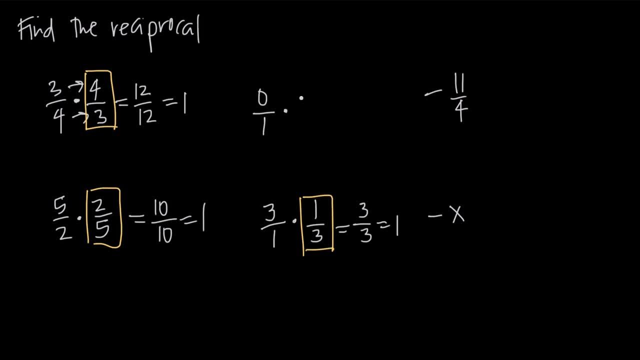 still 0.. Now I have a fraction. I just multiply by the reciprocal, which is what I get when I flip it upside down. so I do 0 over 1.. I get 0, times 1 is 0.. I get 1 times 0 is 0, and maybe. 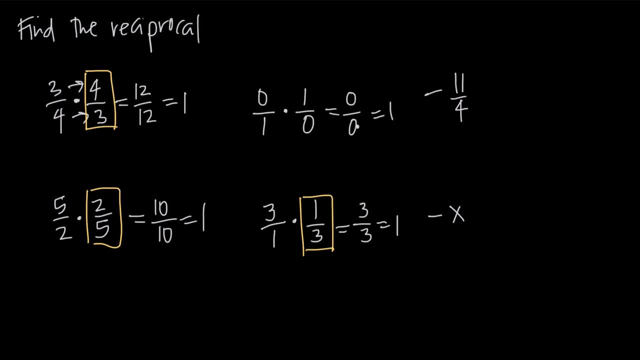 0 over 0 is 1, because anything over itself is 1.. Well, there's so many things wrong with this, it's hard to even know where to start. First of all, we can never have 0 in the denominator, so we can't have 1 divided by 0, because that's undefined, So this doesn't work here. 0 over. 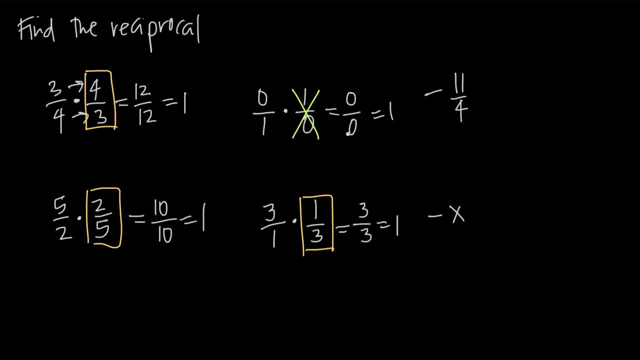 0,. first of all, we can't have 0 in the denominator, and 0 over 0 would be 0. if anything but either, this is going to be undefined also. so what we say is that the only number that doesn't. 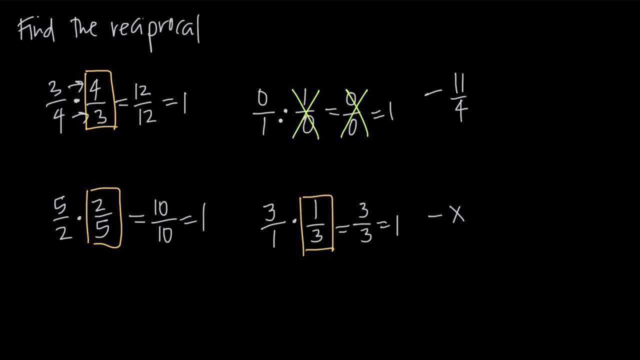 have a reciprocal is 0. Everything else we're going to be able to find a reciprocal for, but there is no reciprocal for 0.. What about negative numbers? Here we have negative 11 over 4, so we just flip the numerator and the denominator and we say 4 over 11.. If I 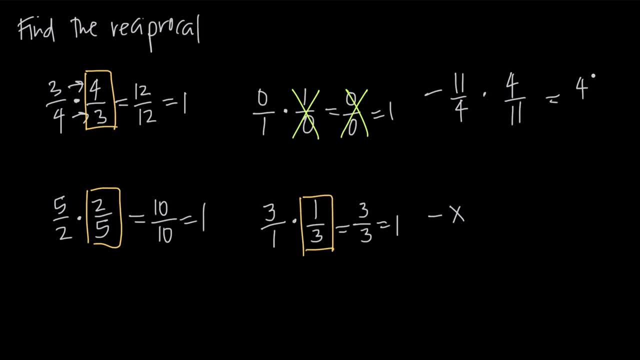 multiply straight across. I'm going to get 11 times 4,, which is 44.. I'm going to get 4 times 11,, which is 44, but I have this negative sign out in front, so I would put a negative. 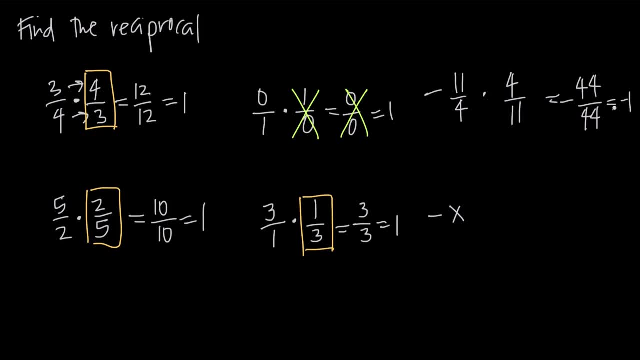 sign out in front and I would get negative 1.. But remember, the reciprocal is what makes this value here: positive 1, not negative 1.. So in order to find the reciprocal of a negative number, not only do we have to flip the numerator and the denominator, but we also have to include. 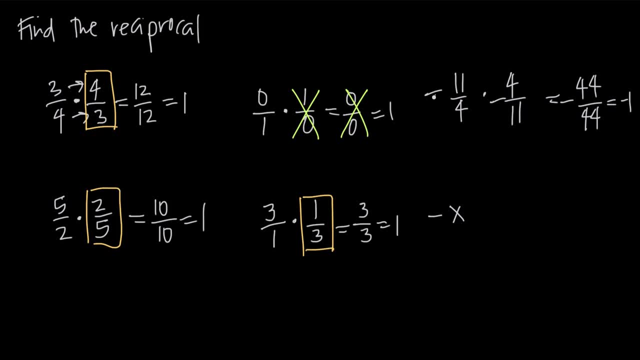 a negative. If I include a negative here with my reciprocal, then I get a negative times. a negative gives me a positive and I end up with positive 1. So then my reciprocal is negative 4 over 11.. Exactly what I get when I flip the numerator and denominator and keep the negative sign.